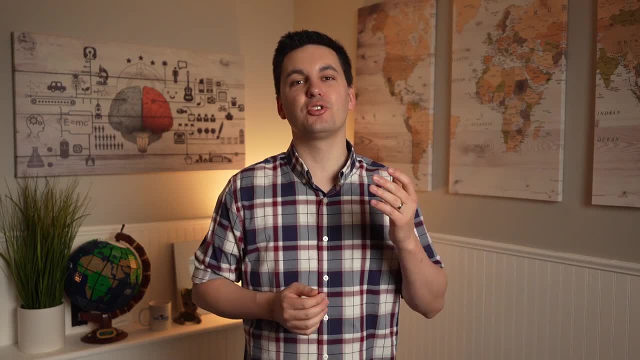 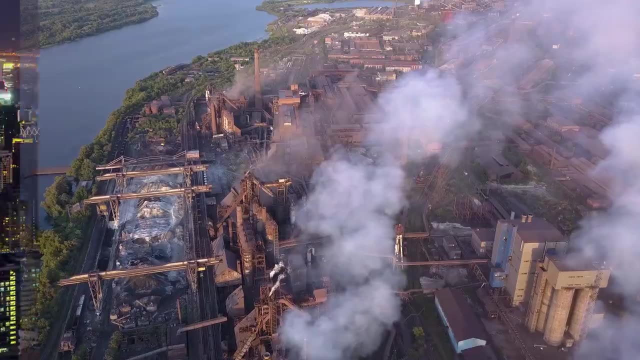 their wants and needs as well. Today, there are many concerns about the current rate in which our resources are being used and depleted. As more countries continue to industrialize and modernize, we continue to see new global challenges emerge. On one hand, we can see that, as countries, 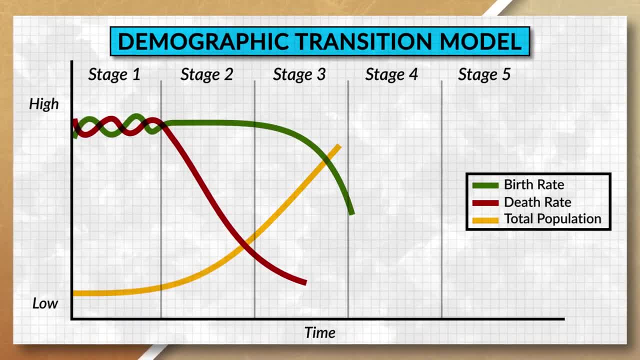 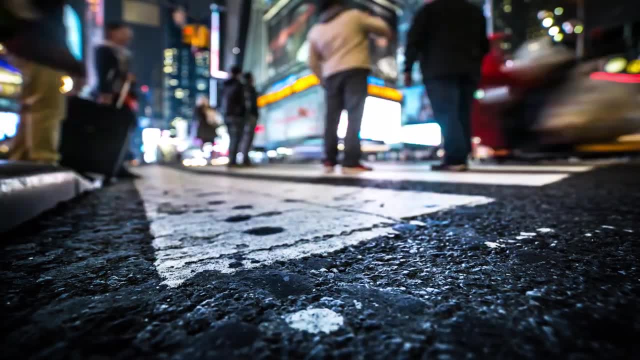 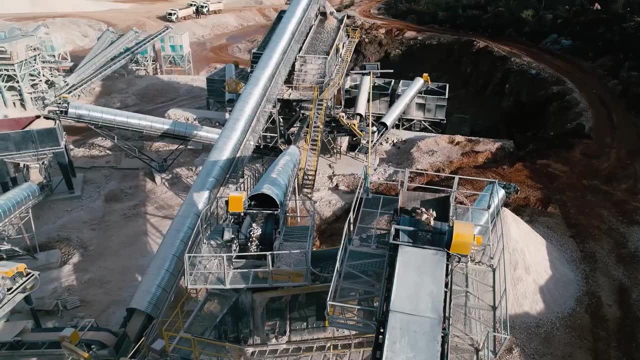 progress in the demographic transition model, they start to see their growth rates shrink. This can reduce the overall pressure on the local environment. But on the other hand, as countries continue to develop economically, they start to consume more fossil fuels, become more focused around consumerism, have higher land and resource usages. 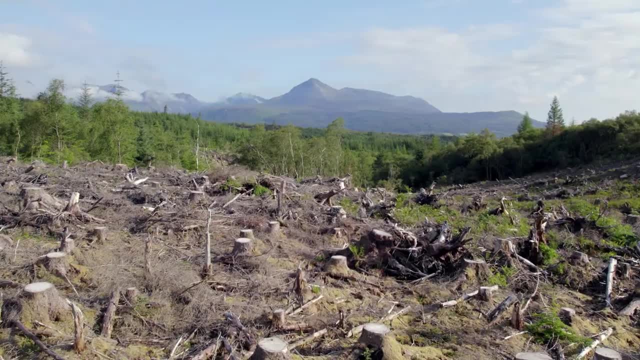 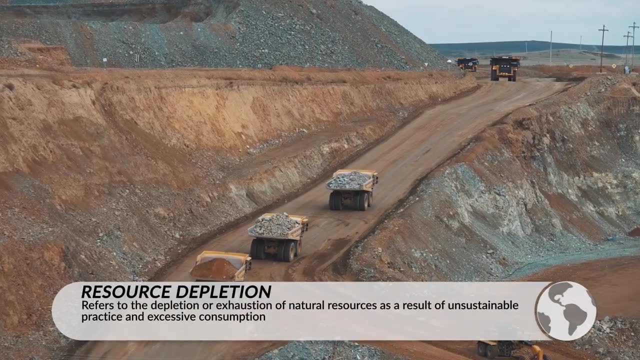 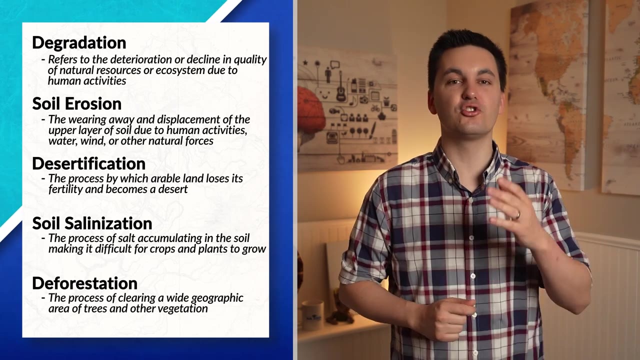 and also see increased energy demand. All of this often leads to resource depletion as the amount of natural resources needed by a society increases, resulting in environmental degradation. as natural resources start to become depleted and exploited, We can also see land degradation occur due to soil erosion, desertification, soil salinization. 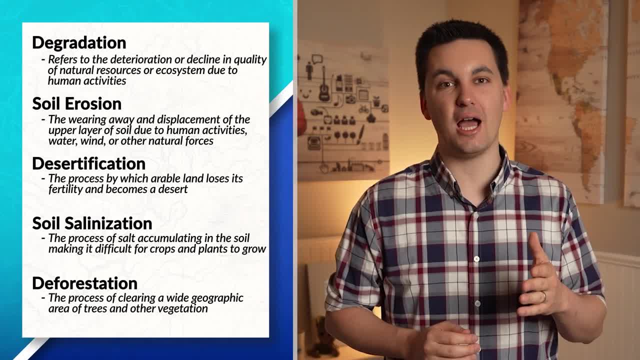 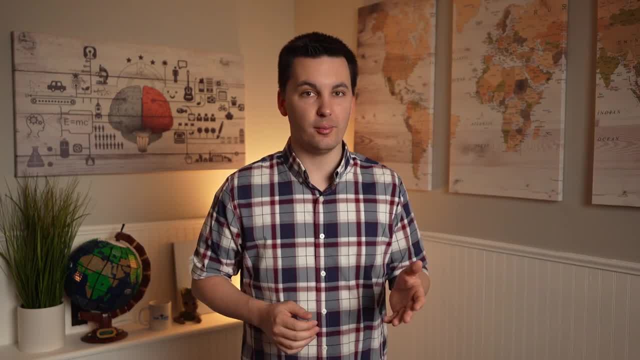 or deforestation- All concepts we talked about in our Unit 5 when we looked at consequences of agricultural practices. In fact, we can see that when societies do not protect the natural environment and continue to abuse it, the consequences can be quite severe. For example, 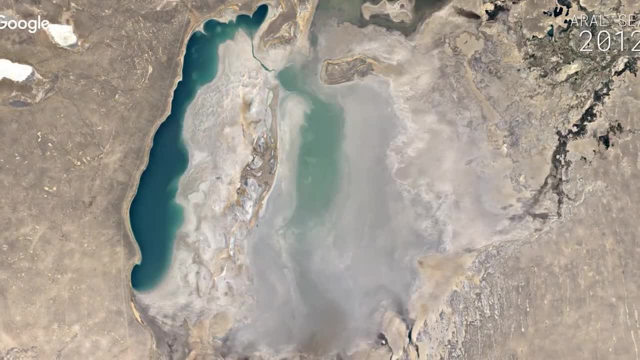 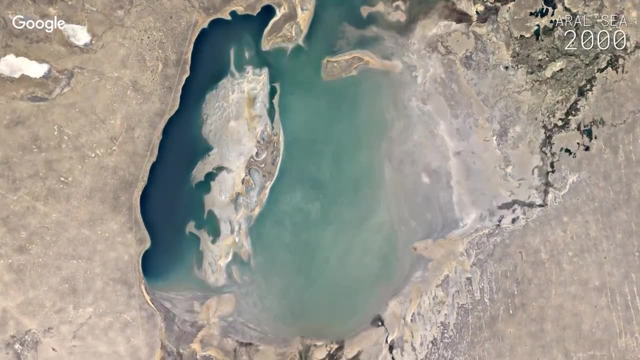 we can look at the Aral Sea, which dried up during the Soviet Union. The Soviet Union diverted the rivers that flowed into the Aral Sea to help with the irrigation of crops, which led to the majority of the sea disappearing. This destroyed the economies of the local fishing. 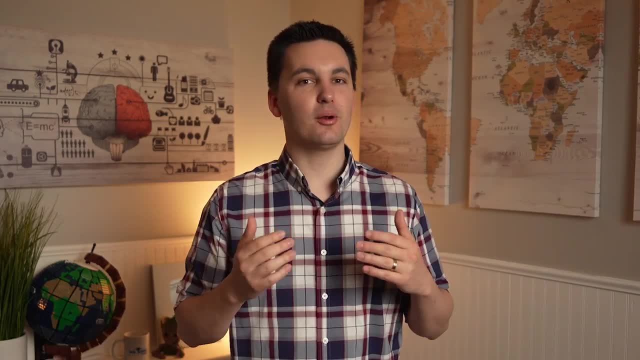 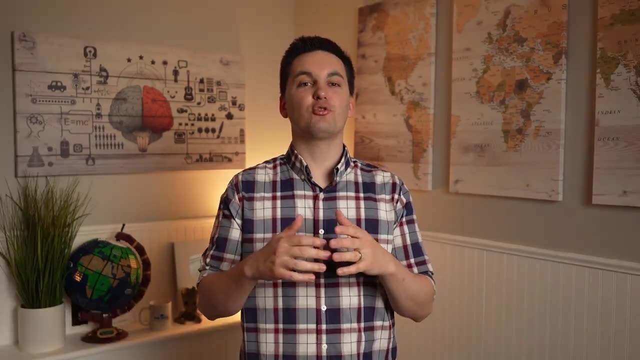 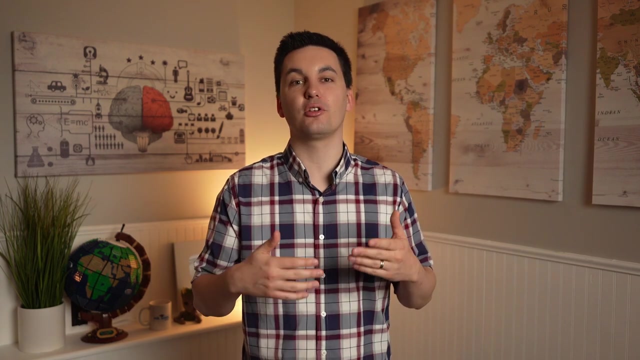 villages and turned the once prosperous sea into a desert. Here we can see human environment interaction, as the environment and society influence one another and how sometimes the consequences can be negative. Now, as countries around the world continue to develop economically, we can also see their citizens continue to see an increase in their overall consumption habits. 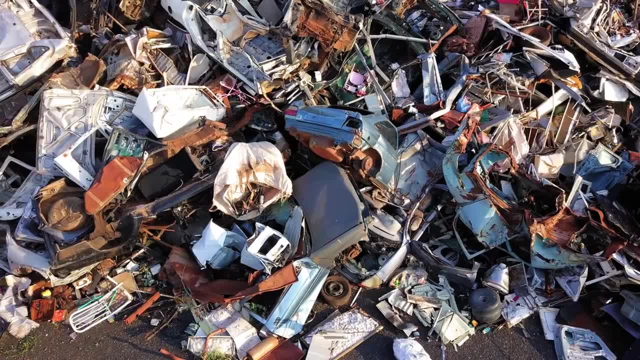 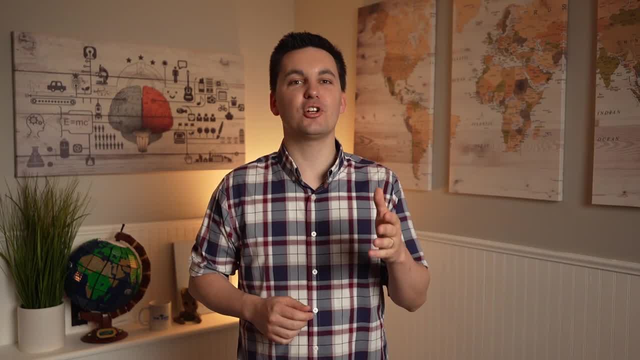 all of which increases the amount of air, water and soil pollution in the environment and leads to more landfills and more wasted resources, along with increased greenhouse gas emissions. In fact, today we can start to see the effects of climate change around the world when looking 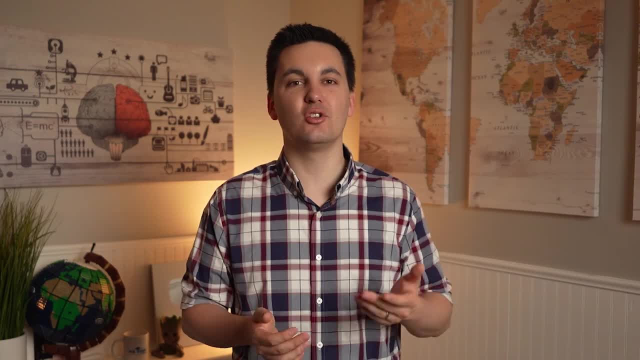 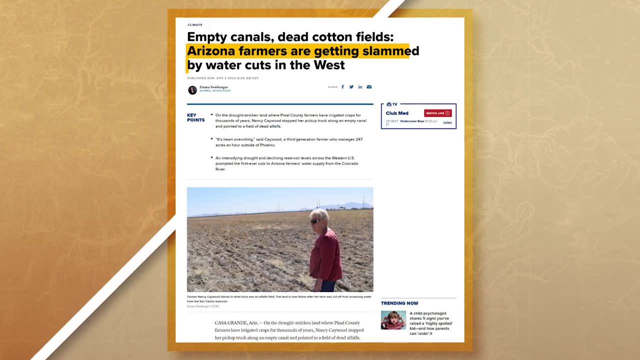 at regional water sources. Water shortages are now impacting the western region of the United States and many other countries as well, Such as in Arizona, where farmers are experiencing water cuts due to a decline in the reservoir levels. across the United States, Farmers that have 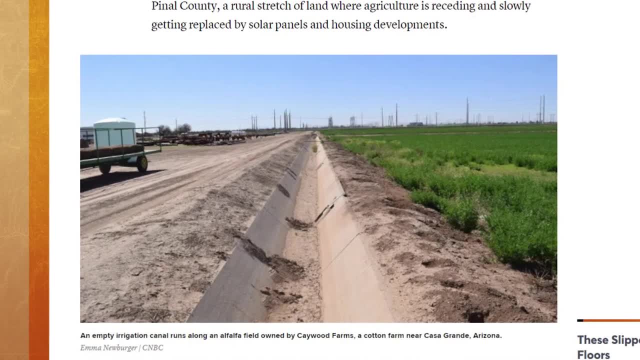 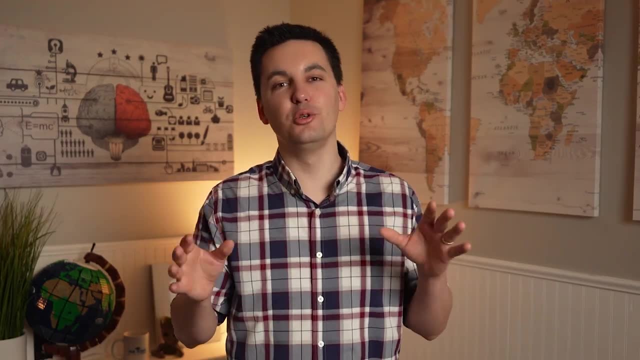 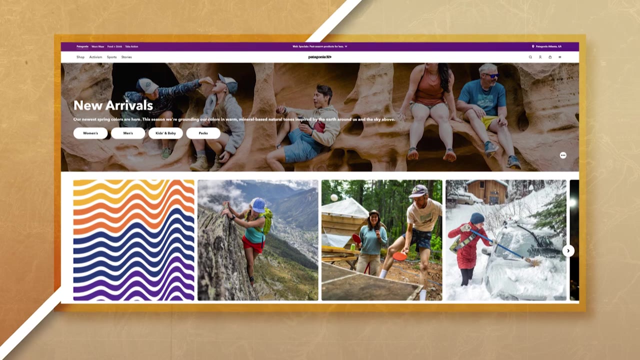 irrigated crops for generations are now facing drought conditions, empty irrigation canals and water shortages, which reduce their ability to produce their products. Now it isn't all gloom and doom. Many companies around the world are working to implement sustainable practices in their production, such as Patagonia, which has made sustainability part. 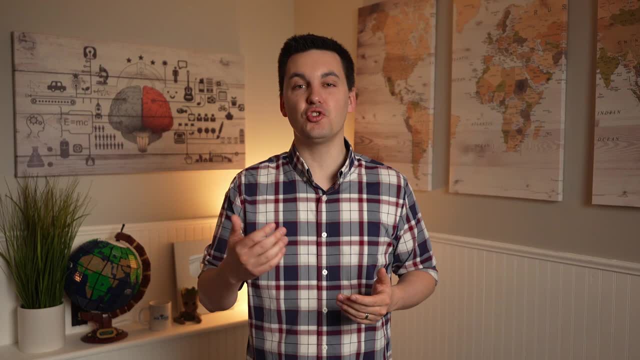 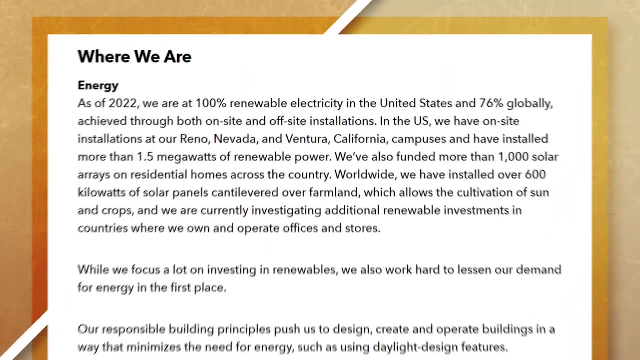 of their business model. The company uses recycled materials such as old garments and plastic bottles in its production and is committed to reducing its carbon footprint. According to Patagonia, in 2022, their owned and operated facilities in the United States used 100% renewable electricity. 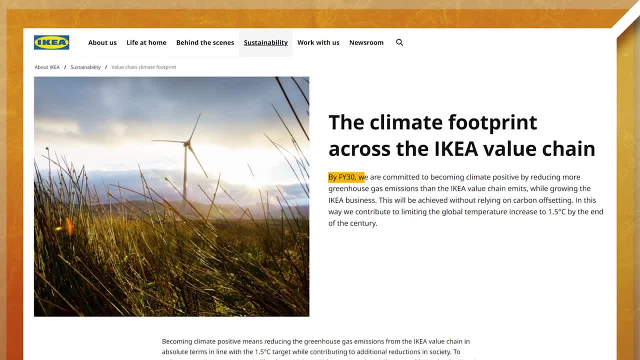 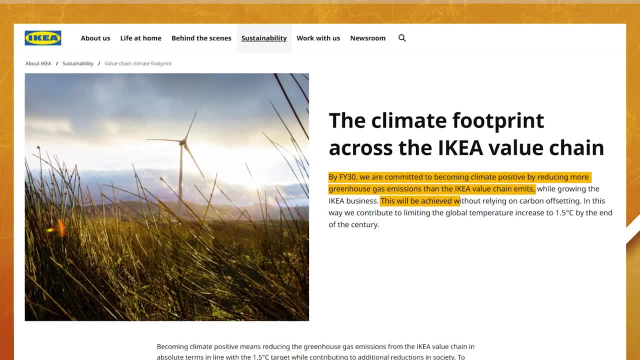 while globally they are at 76%. Other companies, such as IKEA, have created a goal to become climate positive by 2030, which means that the company will remove more greenhouse gas emissions from the atmosphere than it produces. We can also see that countries are seeking to do their. 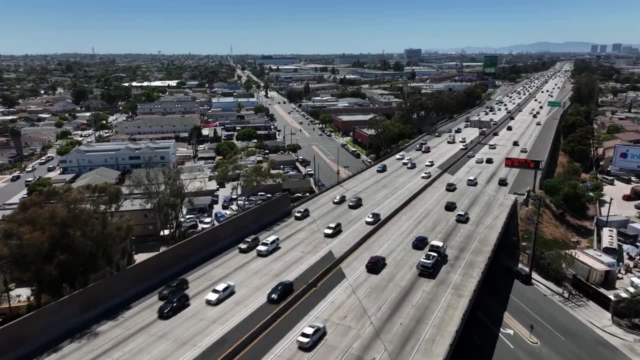 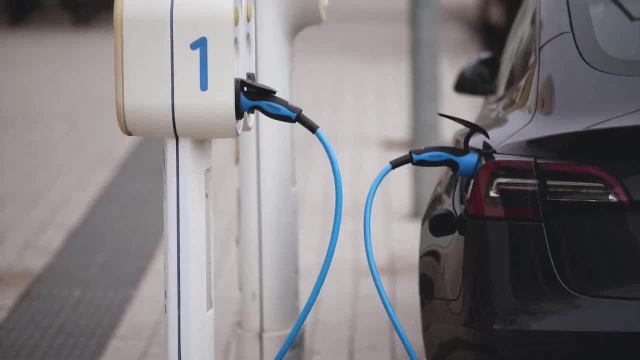 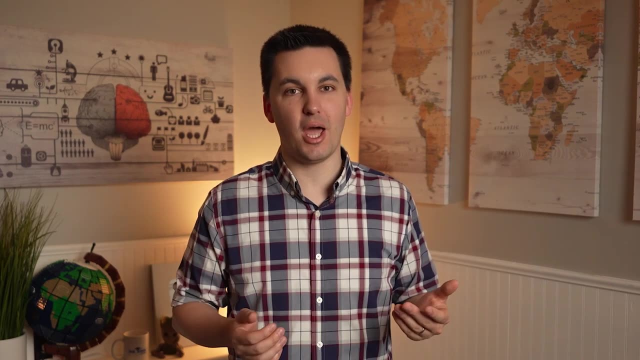 part as well, by supporting green energy, reducing urban sprawl, making recycling programs more accessible, promoting carpooling and creating regulations to create more energy efficient cars and appliances- All of which is just scratching the surface- Another way in which societies can reduce the environmental impact of consumers, while 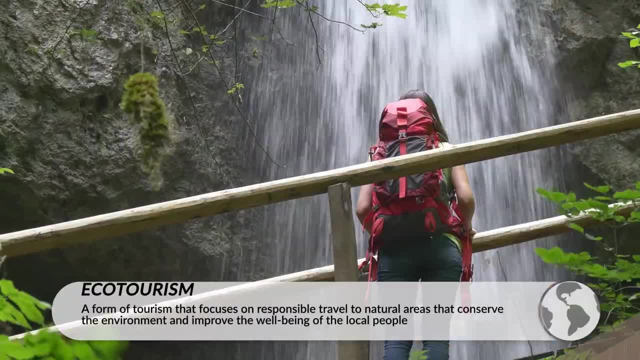 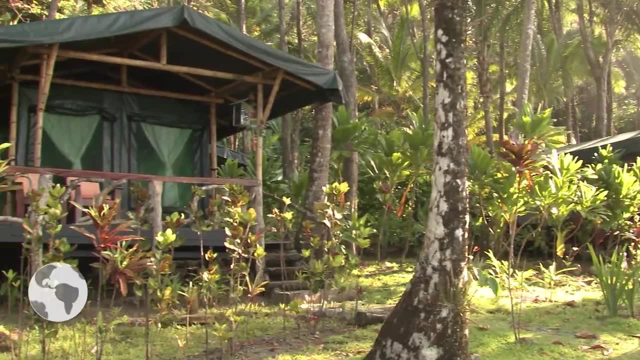 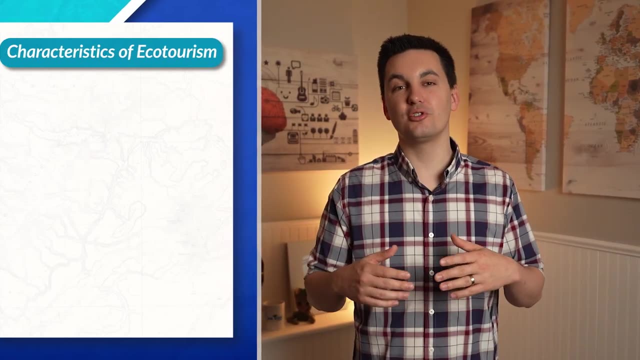 promoting young people to foster their minimal financial problems is by promoting ecotourism, which is a form of sustainable tourism that supports both the local environment and people. The main goal of ecotourism is to promote conservation of natural resources, while also promoting an enjoyable and educational experience for its visitors. 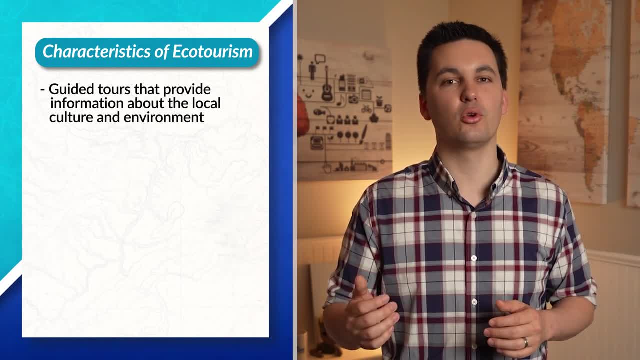 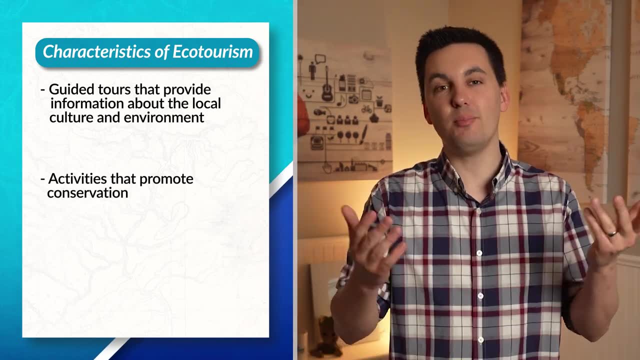 Ecotourism tradition randomly involves participating in guided tours that provide information about local culture and environment. also participating in activities that promote conservation, such as wildlife watching, and by participating in tours that are often run by small-scale, low-impact operations. 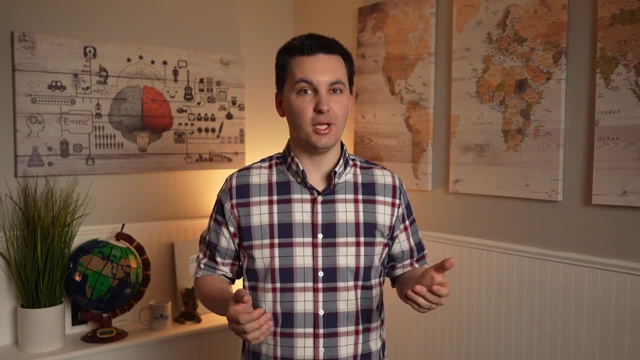 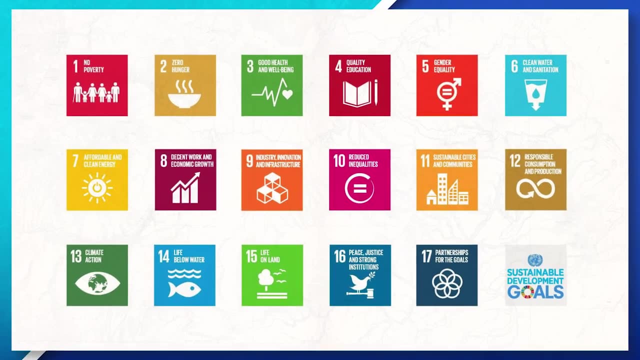 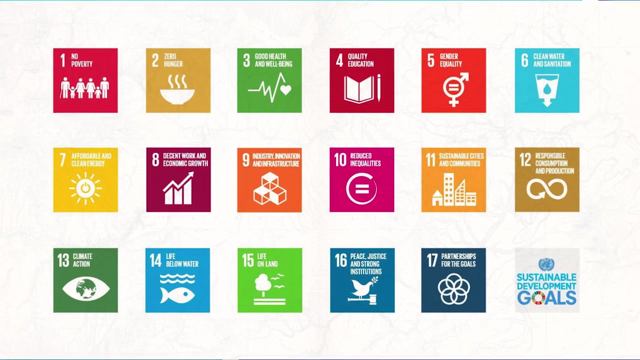 Lastly, we can also see that countries can promote sustainable development by following the Sustainable Development Goals created by the United Nations. If you notice, these goals consist of a variety of different topics that we have talked about throughout this entire course. We can see that there are 17 different goals that the UN has created, with each goal focusing 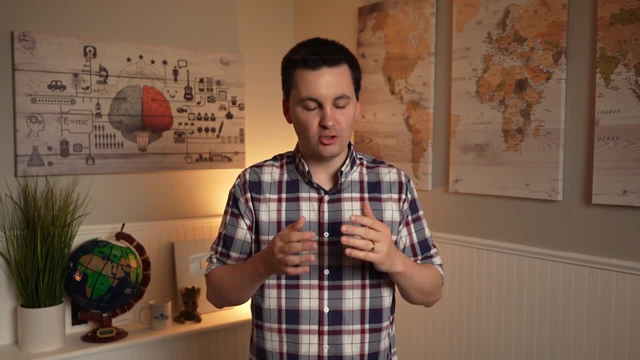 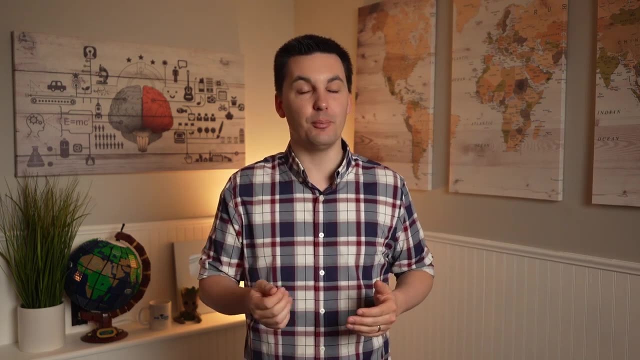 on a different aspect of society. Now don't worry about memorizing each goal. Instead, focus on how these goals connect with not only the topics in this class, but how societies develop and support their people. For example, countries that seek to focus on reducing and removing poverty will often